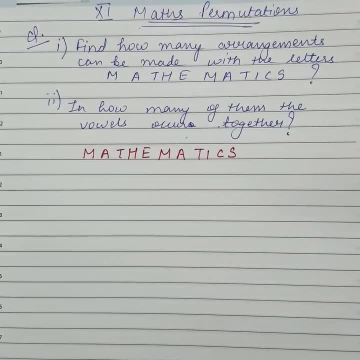 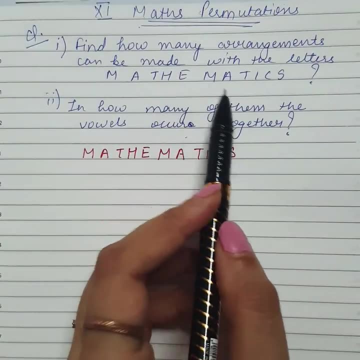 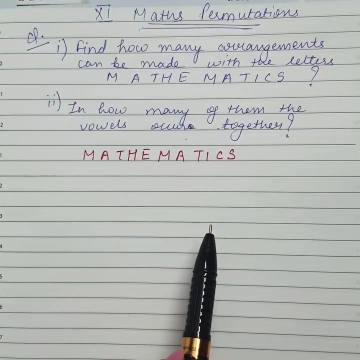 Hello everyone. So in my previous video I asked about this question: Find how many arrangements can be made with the letters of the word mathematics and how many of them the vowels are occur together. Some of you have given correct answers. Congratulations to them. Let us see those who have doubts. 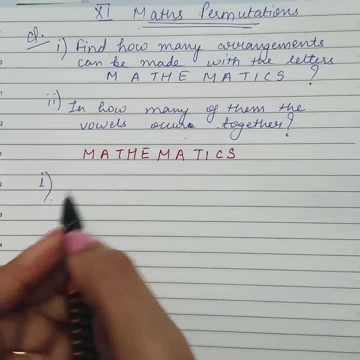 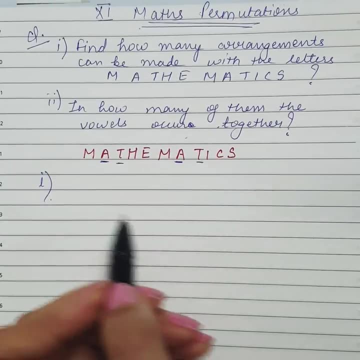 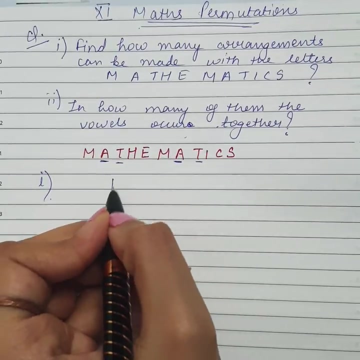 Now see, first of all, for the first part, how many total arrangements. For total arrangements: as we can see, the letters are repeating. So first of all count all of them: 1, 2,, 3,, 4,, 5,, 6,, 7,, 8,, 9,, 10, 11 are there. And now the repetitions. 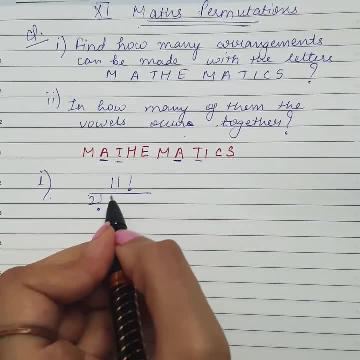 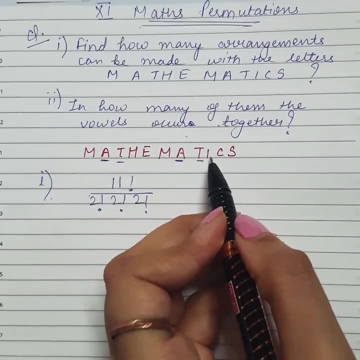 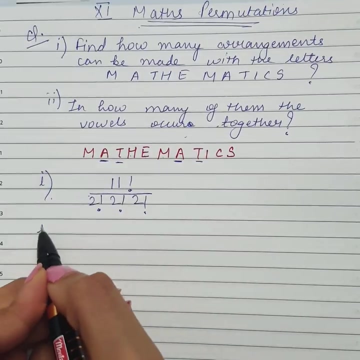 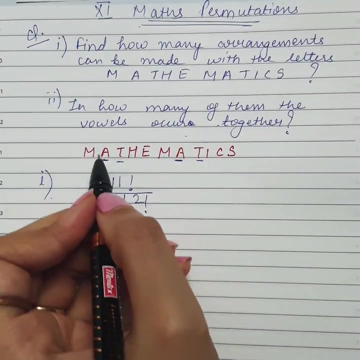 M is being repeated 2 times A, repeating 2 times T, repeating 2 times H, no, E, No, I, C, S, No. So this is how we are going to find out, For second part, in how many of them the vowels occur together. Separate all the vowels. We have the vowels A, E, A, I. 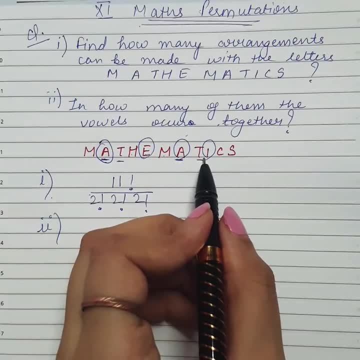 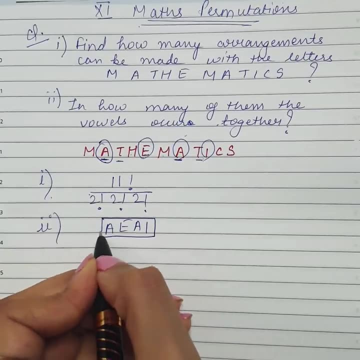 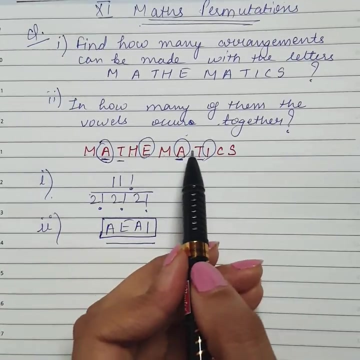 4 vowels are there. For all the vowels to occur together, enclose them as a single letter. Now, this is a single letter. How many other letters are left? 1, 2, 3, 4,, 5,, 6, 7.. 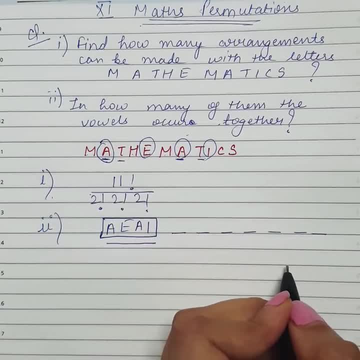 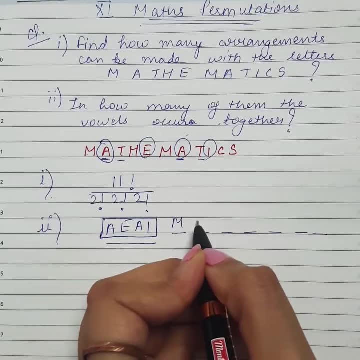 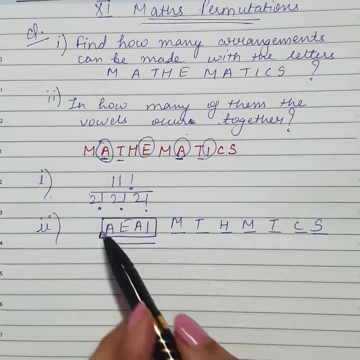 1,, 2,, 3,, 4,, 5,, 6,, 7.. So total 8 alphabets. we have 7, this M, T, H, M, T, C, S, And 8th letter is this complete box. 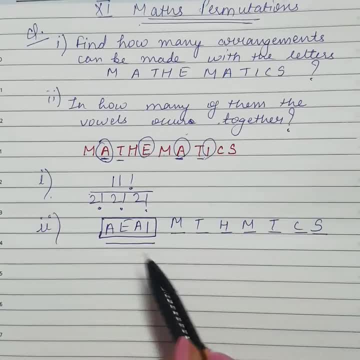 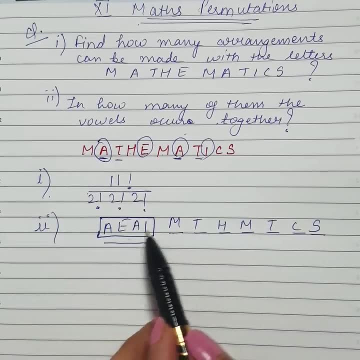 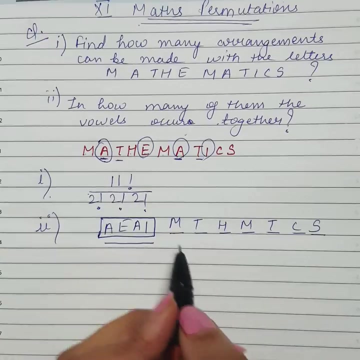 We are counting all of them as one alphabet And then later we will find out the permutations of the box also inside, Because combinations are also possible inside Double A, E, I or E, A, I, A, So many are possible. 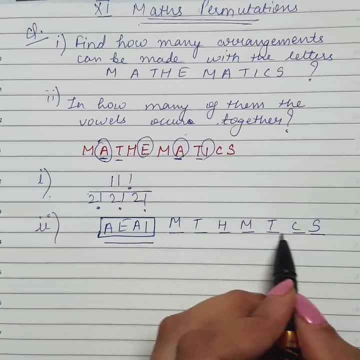 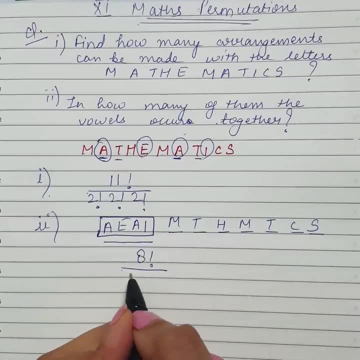 So first of all, all over, we have 1,, 2,, 3,, 4,, 5,, 6,, 7,, 8.. So now the permutations will be: we have repetitions. M is being repeated, T is being repeated.